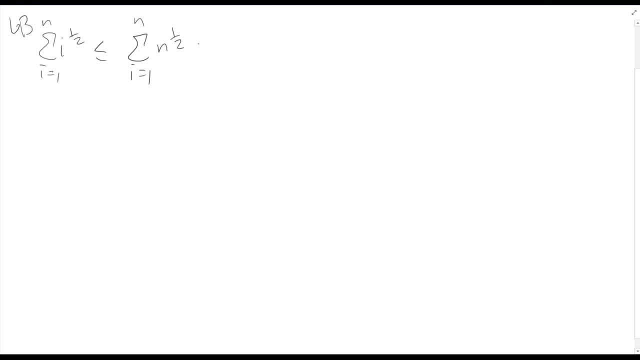 replacing the i with a square root of n, that's an n. basically we get this term here, And then we can complete our math pretty simply. here The n to the 1 half comes out front and we have a very easy sum to compute. 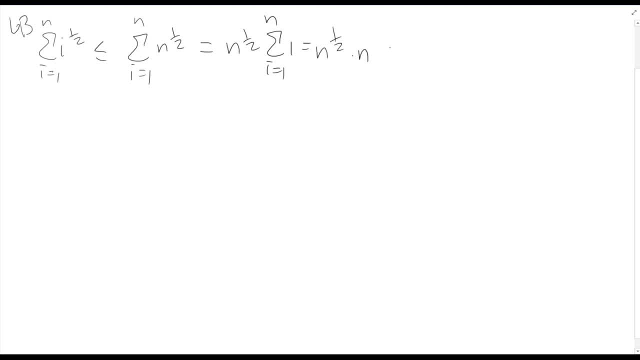 We get n to the 1 half times n, which is n to the 3 halves. And again that's a really good guess for our bound n to the 3 halves. And again we've shown Big O with our upper bound here and remember our B out front. here is a 1.. 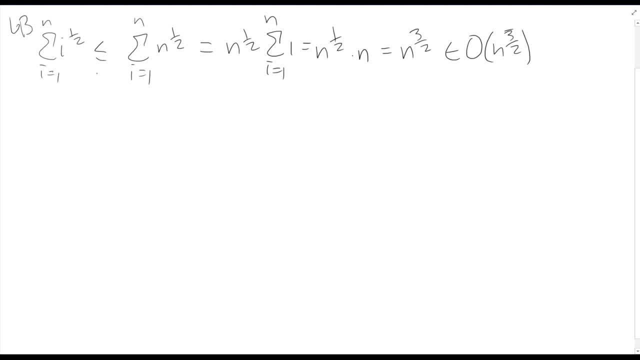 So we've applied the definition of big O with the less than or equals to B times n to the 3 halves. So we've shown big O here. So now we want to do big omega, and big omega means we're going to do our lower bound. 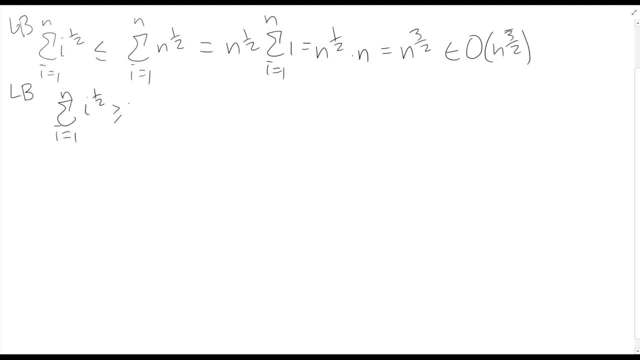 So we're now looking for the lower bound with a greater than or equal to. And again, if we just use the binding, the term technique here, plugging in the 1 here for our i, we'll get 1, well, the square root of 1.. 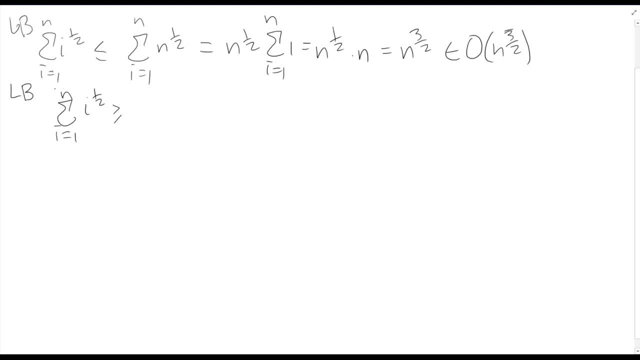 We're actually going to do a little better than in our previous example. We're going to end up with an n total, But our n again doesn't match our upper bound. We need to match n to the 3 halves, and so that's not a tight bound. 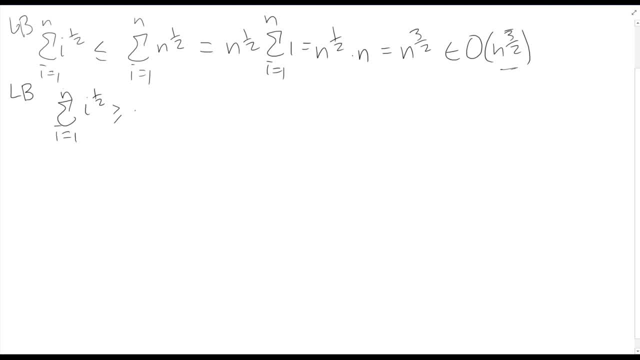 So we definitely need to use our other technique, our splitting the sum technique. So I do want to use the splitting the sum technique And so remember, what we're going to do in the splitting the sum technique is we're going to replace the whole sum, or approximate the whole sum, with half the sum. 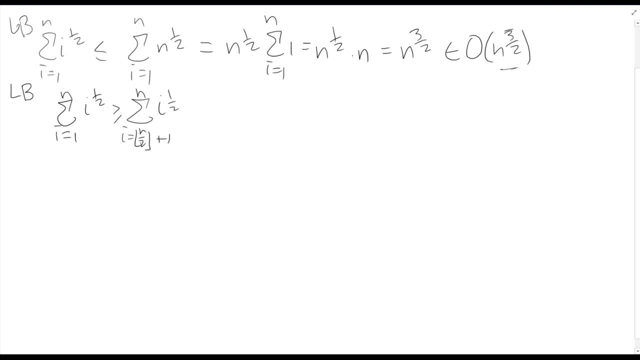 So instead of starting at 1, we'll start around the middle point, the floor of n over 2 plus 1.. And again I've chosen this point. the first half of the sum up to the floor of n over 2, we've thrown away. 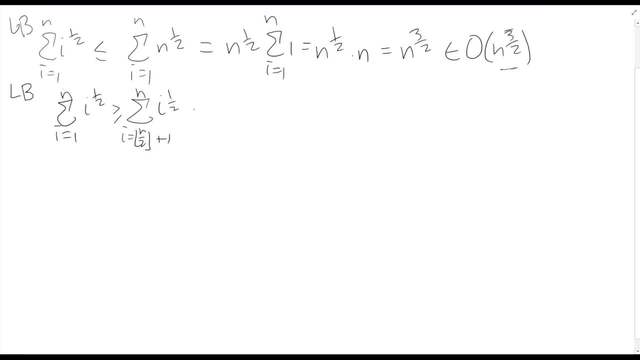 I've chosen this point. The plus 1 is actually going to cancel out with a minus 1 in a little bit, which makes it sort of nice. That's why We're actually going to keep it around instead of maybe trying a different point to split. 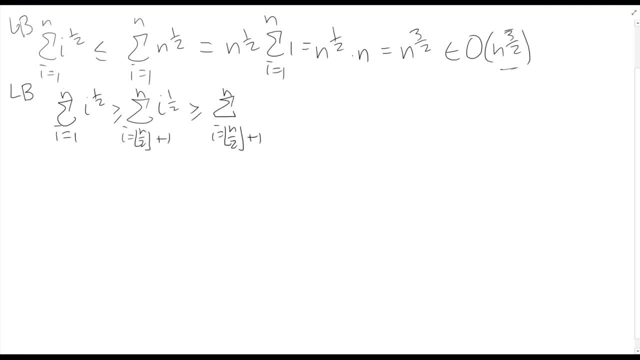 All right. so, continuing on here, we're now going to under-approximate, or we're going to use the binding, the term technique to replace our i here with this value, the lowest it is, Again keeping in mind that the square root of i is an increasing function. 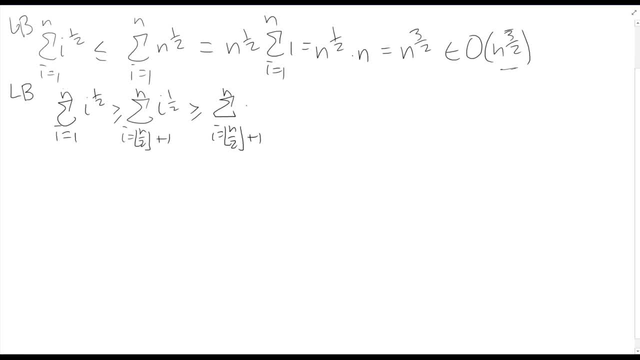 So the smallest this sum gets is when we have the first value. So I'm going to write this here in brackets. All right, now again, that looks a little bit nasty. We've got some stuff inside of a square root, but trust in the math. 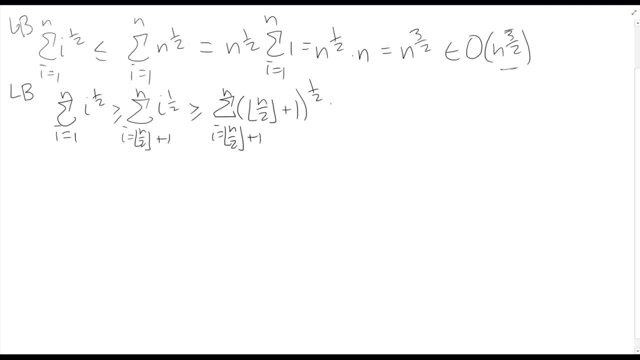 And it's hopefully going to cancel out and make things a little bit easier in a second. So again, two steps of approximation here. First one: splitting the sum, replacing all the terms with half the terms. Second step: we're taking this i and replacing it with its lowest value. 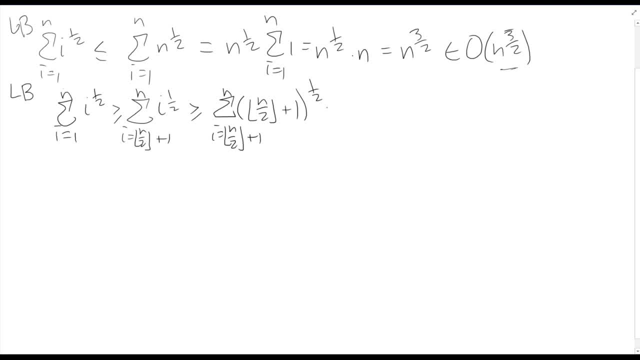 So now we're here. Now, after those two steps, we can factor this out front so we no longer need it, need to keep it there. So we now have all out front. We still have our sum And remember, in our previous video we did determine what this value is equal to. 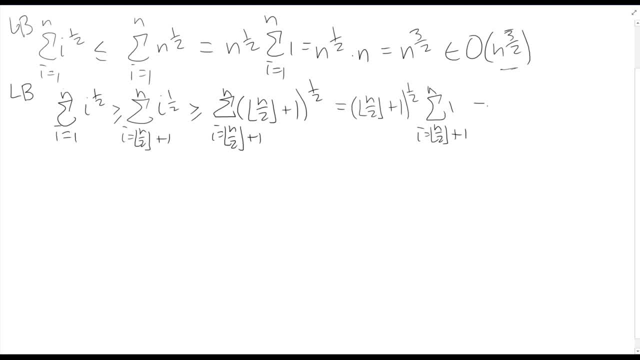 This sum, the whole sum- and maybe I'll just write it here- is just the ceiling of n over 2, the whole sum here. And then what else were we left with? We got this other term that I left here. we got it all to the 1 half. 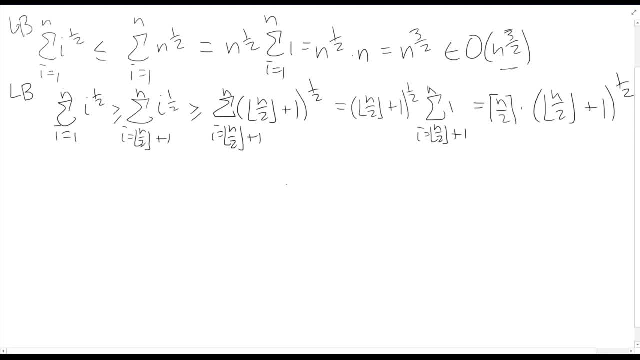 Okay, so not that bad. Let's continue down here. Now again, keeping in mind the notation I used, these two steps were algebraic steps, so I used equals. These two steps were approximations, so I used greater than or equal to. 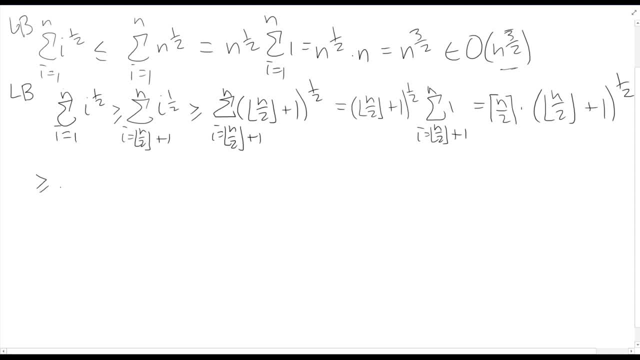 But the next step I'm going to use, I'm also going to do an approximation. I want to start getting rid of my ceilings and floors. Okay, And again here, keep in mind the ceiling of n over 2 is always greater than or equal to n over 2.. 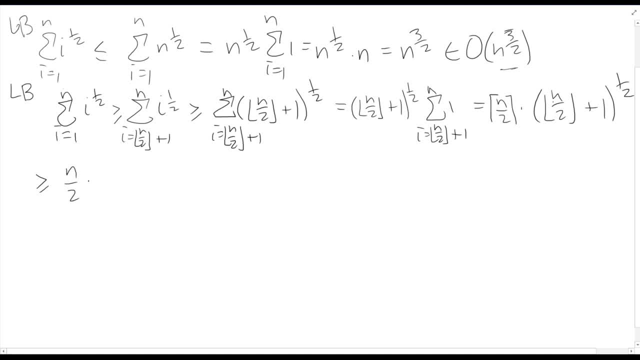 That's just an easy one. We can drop it off on this direction. But the floor of n over 2 is greater than or equal to n over 2 minus 1.. So the minus 1 is going to cancel with the plus 1.. 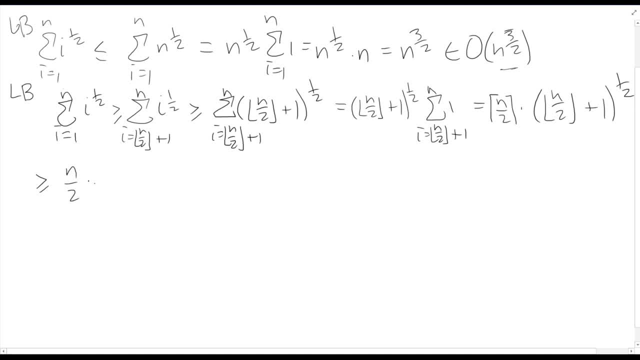 I promised you that was going to happen. So that's going to leave us here with n over 2 to the 1 half. So the final result: So the final result- is n over 2, the whole thing to the 3 halves. 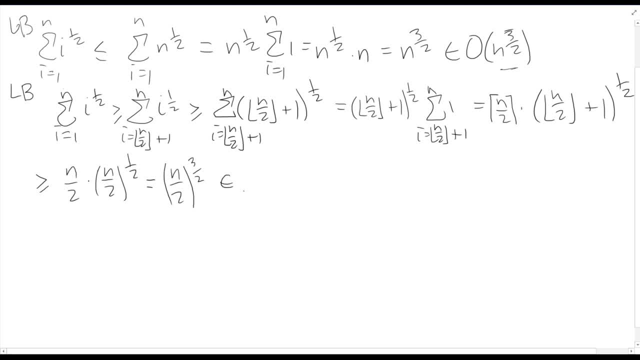 Now notice this is big omega now of n to the 3 halves. The value we have here. it's maybe a little bit harder to see, but it's 1 over 2 root 2, or 1 over 2 to the 3 halves is the value of a that we have. 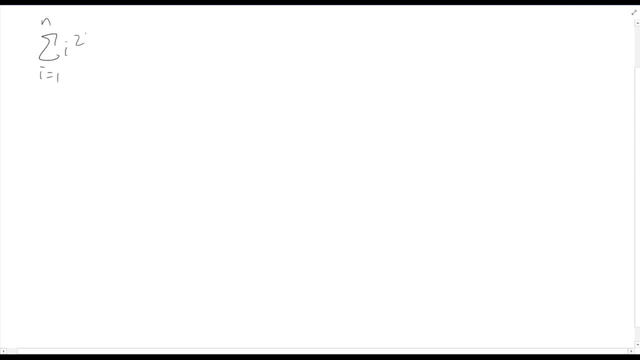 In our proof for big omega. All right, I'm going to do another one here. The sum from i equals 1 to n of i squared. And again, maybe I'll start with my upper bound here. Some of you maybe, if you've already studied your summations in a little more detail. 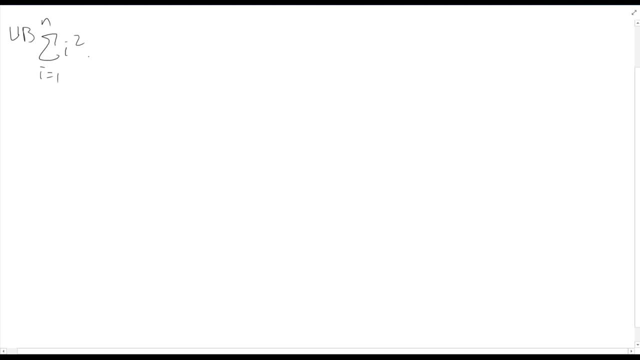 you. probably you might already know what this is equal to. I must confess, I know that it has a closed form, but I've never actually memorized it. I probably could make a guess at it right now. I'll write down some numbers. 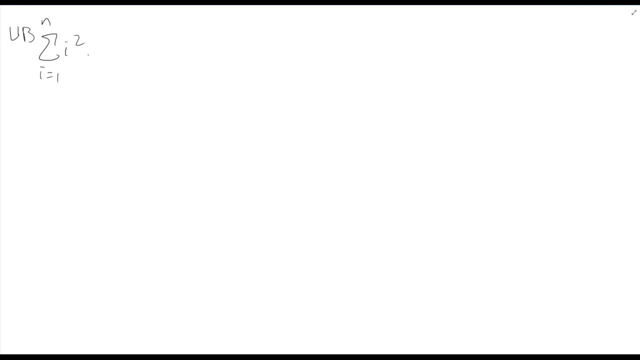 I know there's a 3,, a 2. And a 6 in there. I might mix up which order they go, But that's part of the reason why I don't know what it is is because, in my as a computer scientist, 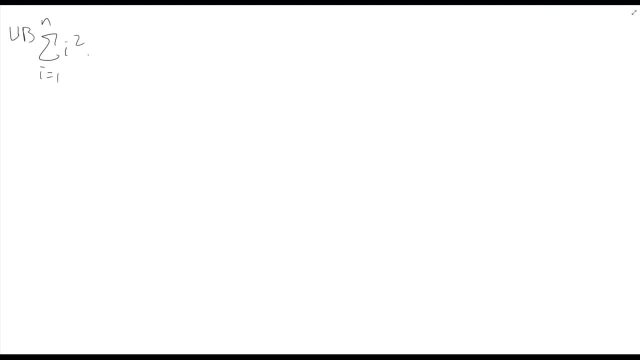 I rarely need to know what it exactly is equal to. More often than not, I'm okay with just knowing what an upper and a lower bound is, And I already know what my upper and lower bounds are on it, So that's probably why I've never committed it to memory. 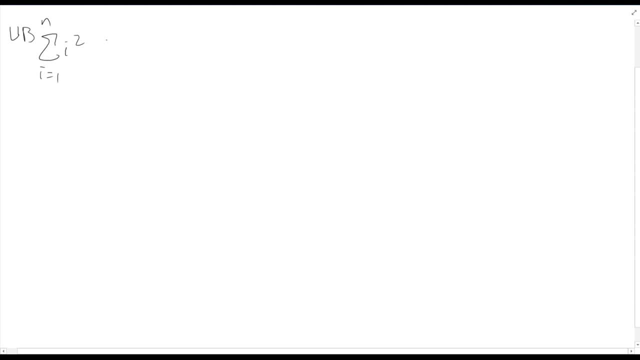 So let's maybe go through it ourselves, And then maybe we will not need to commit it to memory either. So I'm going to do the upper bound first, And here we are. following the same technique. I'm going to replace that i squared with an n squared, making it as large as I can. 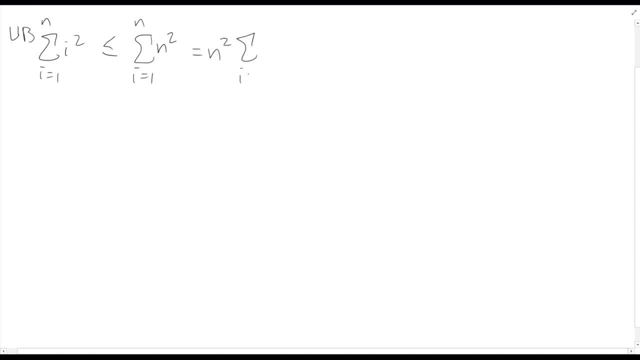 And then we're just going to get some pretty straightforward steps now that we've practiced a couple times. now, Okay, Again the n? squared has come out front. We left off with a 1. And then obviously that whole thing is just going to collapse. 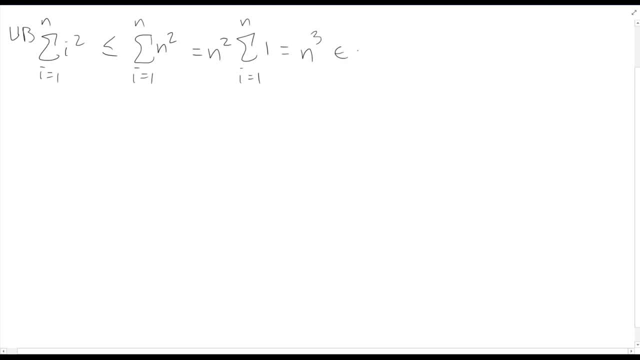 This becomes another copy of n. So we're up to n cubed now And again. maybe n cubed would be a good guess. Hopefully, if you've been practicing along and following along here, you're starting to see a pattern. 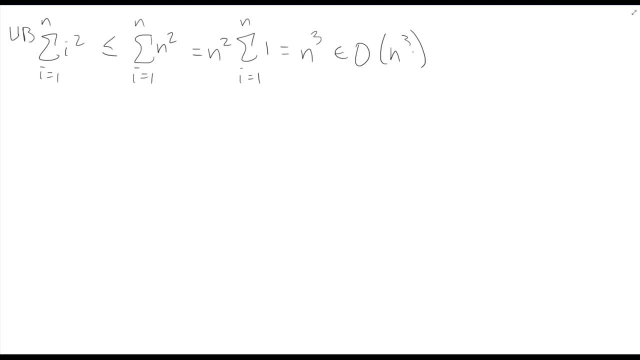 And maybe you can go ahead and start filling in that pattern yourself in your own computer, So that you have maybe some more intuition about what you're going to see. So again, we want to tackle this problem, But on the lower bound now. so on the lower bound. 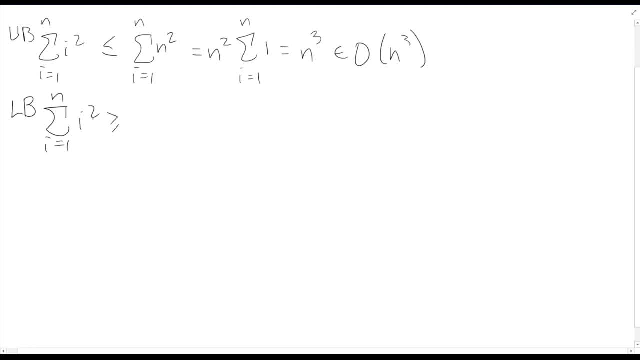 we're going to be doing greater than or equal to, And again I need to use splitting the sum. Let's just verify that. if I plug in my 1 for all these terms here, they'll all just turn into 1's. 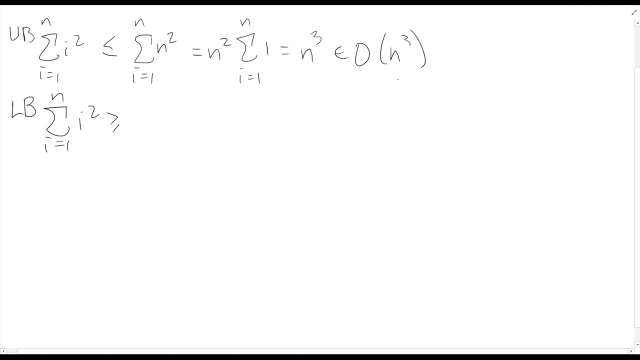 So we'll actually only get n, And my lower bound again will be n. Well, n is not a good lower bound for n cubed, That's not a tight lower bound. We want one that matches. So if we want one that matches, we are again probably going to have. 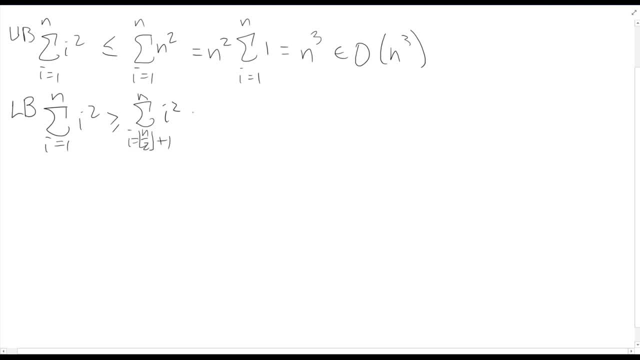 to use our splitting the sum technique. So let's split the sum Again. that's the first step That makes it possible for us to now under-approximate that term. So my i squared term, going to be careful here. Floor n over 2 plus 1 all squared. 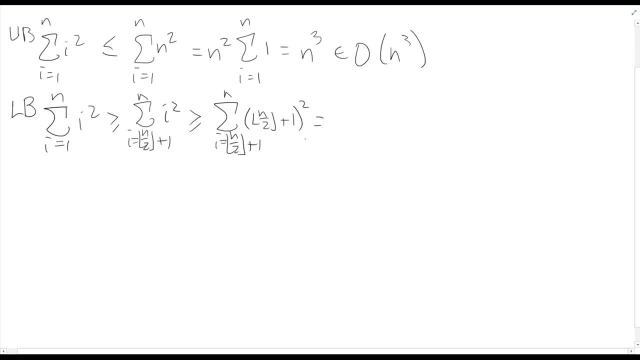 Again, two approximation steps to get to here. Now we need to do a little bit of algebra and maybe one more approximation at the end to get rid of our floors and ceilings. So a little bit of algebra we're going to factor out. 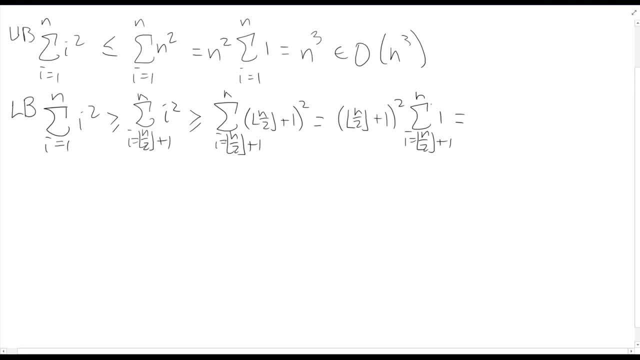 Again. we've now seen this sum three times And again it's the ceiling of n over 2.. And we're left with this term still that we need to bring over. So that's going to be the floor of n over 2 plus 1 all squared. 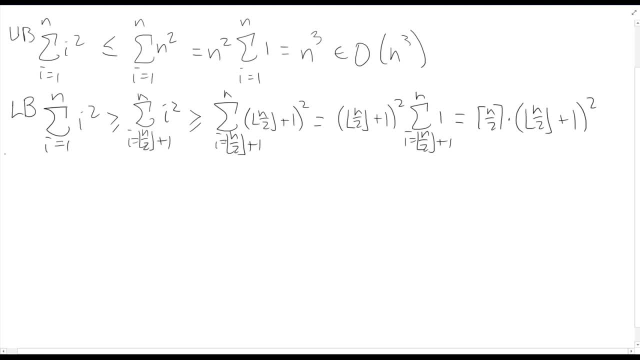 Again. you've sort of got your notes. You can see we've got a very similar pattern to the last example. Okay, continuing on. oops, I put another equals, But this is time for another approximation step where I want to get rid of my ceilings. 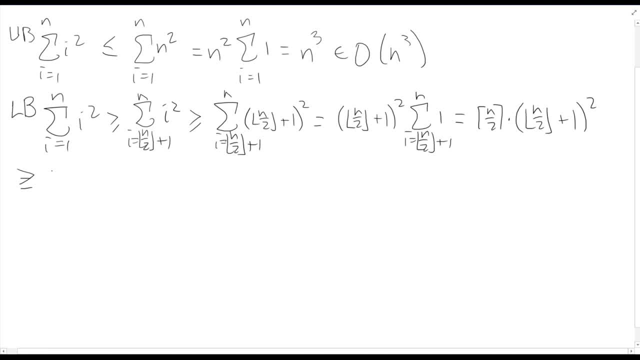 and my floors. So get rid of my ceiling here. Remember, the ceiling of n over 2 is just straightforwardly greater than n over 2 itself. Maybe I'll leave that in brackets, just to keep mine separate. Same thing here: The floor of n over 2 is greater than or equal to n over 2 minus 1.. 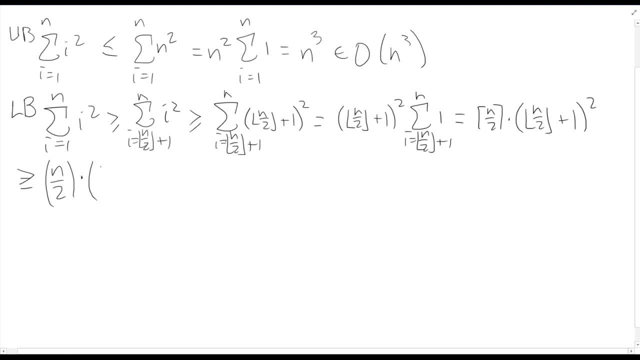 The minus 1 and the plus 1, again cancel out. That's been happening in all our examples. Again, we have an n over 2 here, But this one's really important, So we're going to get rid of that. 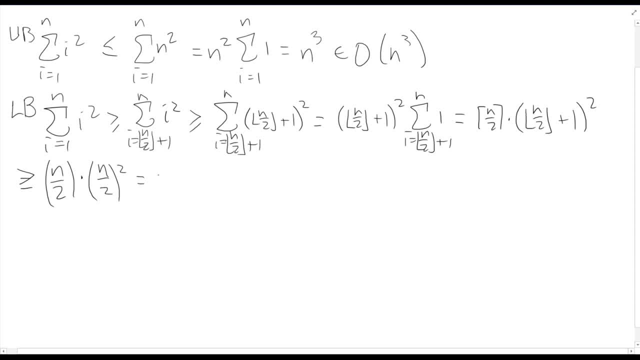 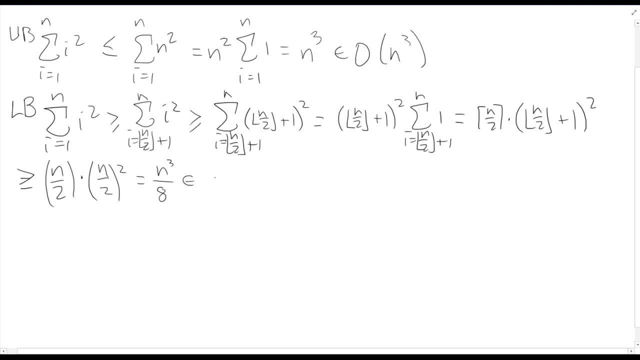 Again giving us our big omega of n cubed. So big omega matches our big O. That's good, Remember? that's sufficient, then the two of them together for big theta. So we've now shown our sum. Our sum is in big theta. 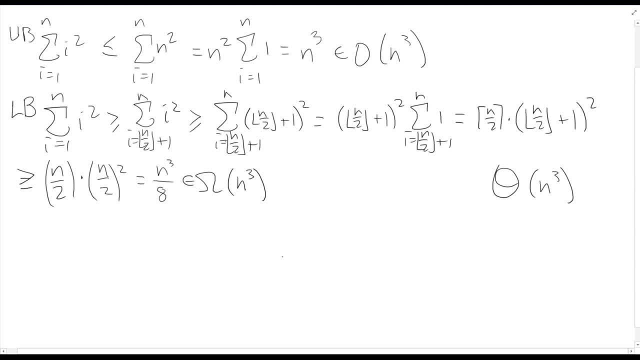 And that's what we're hoping for. Maybe I will finish, because this is sort of an important worth noting, that we've gone ahead and done a proof on this sum. now We did an upper bound, We said that this is less than or equal to n cubed. 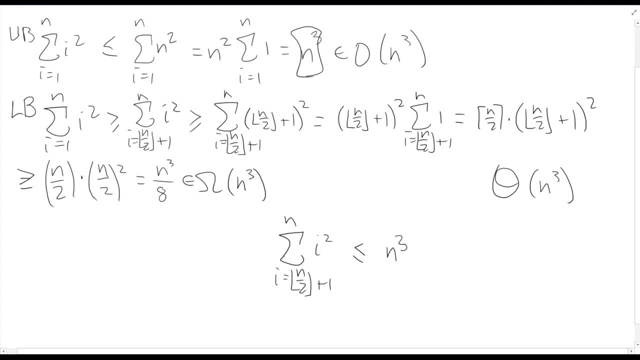 That was the value we got up here, And our value up front was a 1.. And then on the bottom end we still had our n cubed, But maybe I'll write it like this: It's 1: 8.. So we found we've come up with a description. 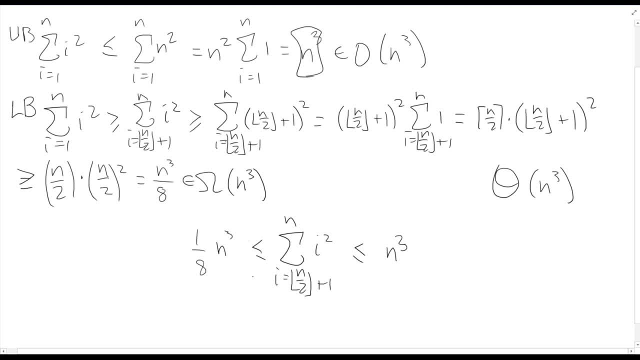 We've come up with an estimation of what this sum is going to be equal to, And maybe it might be worthwhile for us to think a little bit of what that's going to look like. So here I made a cube. Now, this cube if we had n, n, n. and where does my other n need to go? 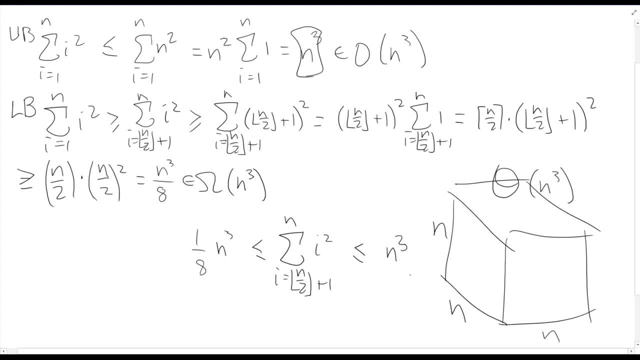 Here. If this is a n by n by n cubed, right, then the volume of that cube is this: Okay, So we're saying the sum, the sum of all these squares that we were interested in, is less than this area. 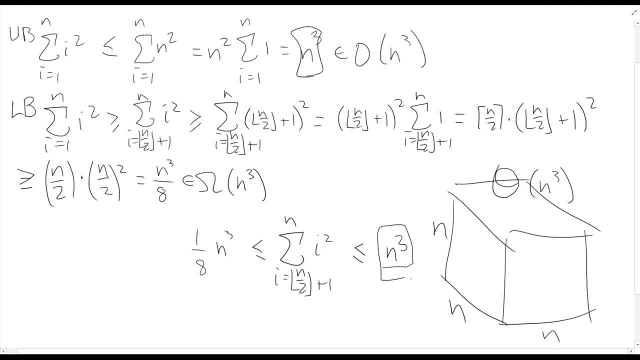 Okay, Now what's 1, 8 of this area? Well, when we're working with cubes, 1, 8, is this little quarter If we, if we split off all our dimensions by, by 1 half here. 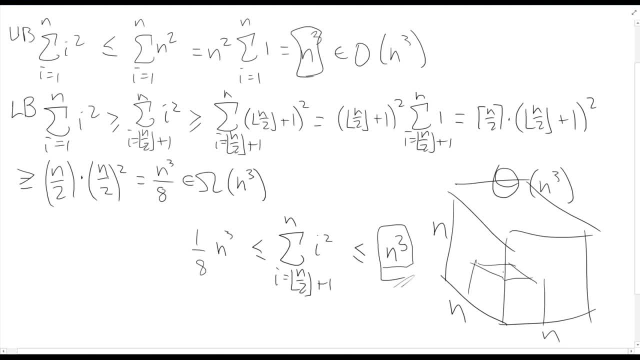 we're actually going to get 8 cubes, 4 on the bottom, 4 on the top. So one of those little ones, that's 1 8th of our n cubed. So the the estimation that we've got here is, if we were. 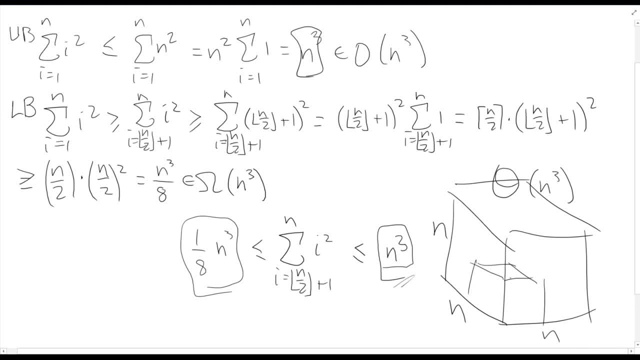 to draw these two cubes. our sum has volume, somewhere between these two And what it is. well, maybe that's a good enough approximation for you, It's good enough for us, It's good enough for us to say it's n theta of n cubed. 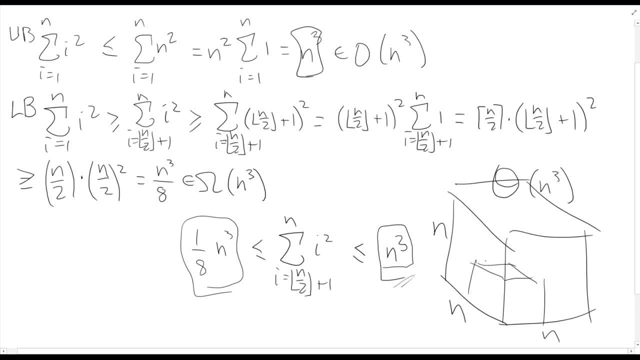 So maybe that's good enough, But maybe we'll want a tighter one, And- and probably in my next video, I will show us a way to get a tighter bound than even this, if we needed it. All right, So I've included this one in here. 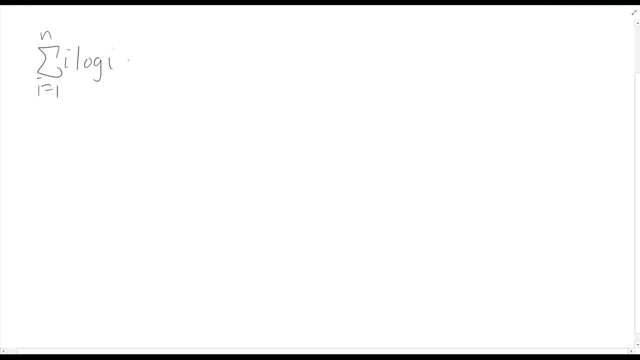 i log i. What would you do if you had to deal with something like this? Now, there's more than one way to tackle this In in a video. a later video, I'm going to show again an example where we need to get a real good. 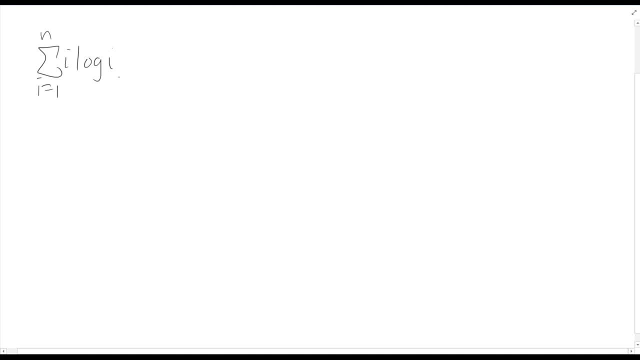 good approximation on this, But I might want to again just practice the techniques we've been using. but maybe let's test our intuition here. We've already done a couple We we just finished one that was: the sum of i equals 1 to n. 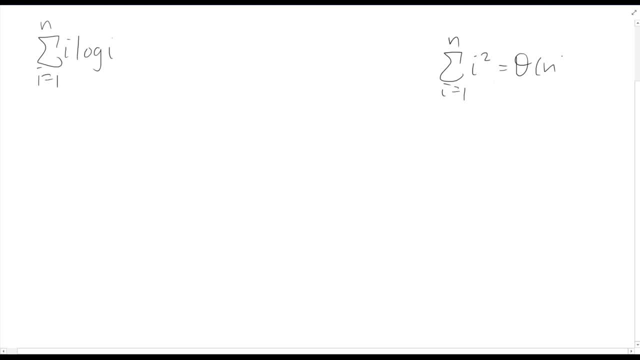 of i squared is theta of n cubed. All right, And we also did. i equals 1 to n of log i squared. All right, And we saw that was theta of n log n. Okay, N log n. So maybe we can kind of come up with a guess for these ones. 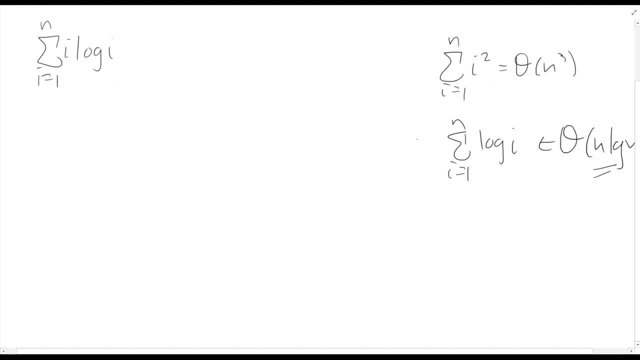 We know the sum of just the i is i squared. So we notice that in this example we got an extra copy of that n popping out. it looks like. Well, in this example we also got an extra copy of n. It didn't show up inside the log. 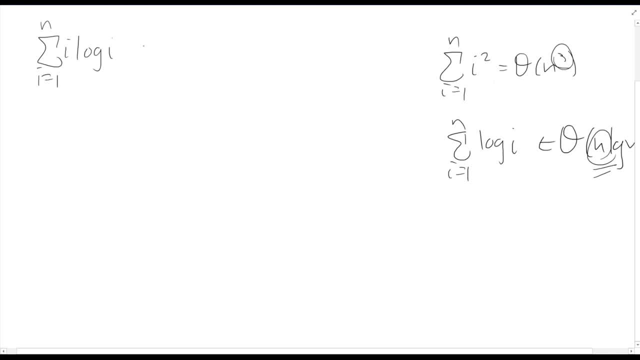 It came up out front. So maybe here a good guess. and here I am just guessing, I'm trying to build my intuition. I might say, hey, this one might be n squared log n. I get an extra copy of n. 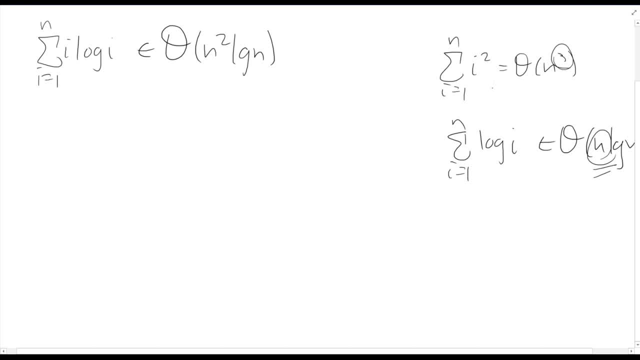 The sum on the outside, gave us an extra copy of n. We've got a guess for what we think this bound might be. Let's see if we can prove it. In fact, the upper bound is not going to be that hard, So I don't need to try too much. 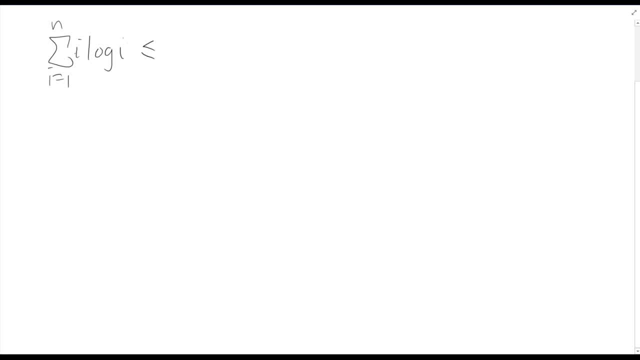 i log n, Or sorry, i log i is still an increasing function, So we can still over-approximate every term by swapping out the i for the n. So let's go ahead and do that, And again, after this step, our term no longer depends on i. 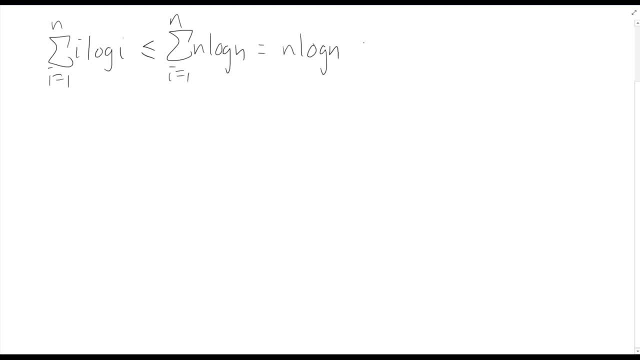 That's the intention, So we can move it out front, leaving a very simple sum which again gives us an extra n. That's what our guess was. Oops, I wrote a 3 there. Let's make that look more like a 2.. 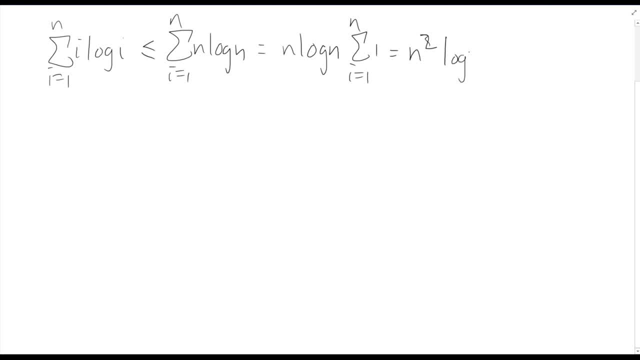 All right. So we're going to do n squared log n And again, that's sufficient for our big O And maybe that's all we're concerned with. A lot of the time that is all we're concerned with. So we get n squared log n. 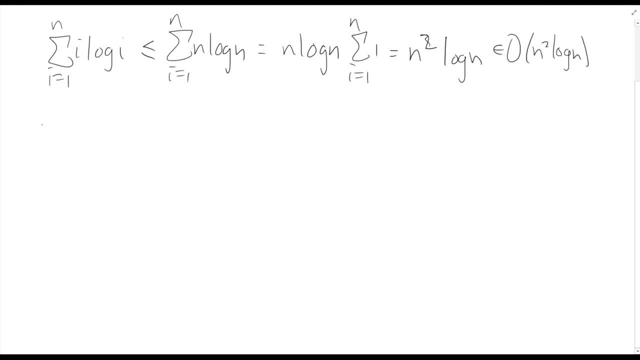 Okay, Now again, if that's all we're concerned with, we're done. Otherwise we'll continue. Now for the next one. I'm going to use the same technique, the splitting the sum and binding the term, But I am going to make it a little bit easier on myself because, frankly, 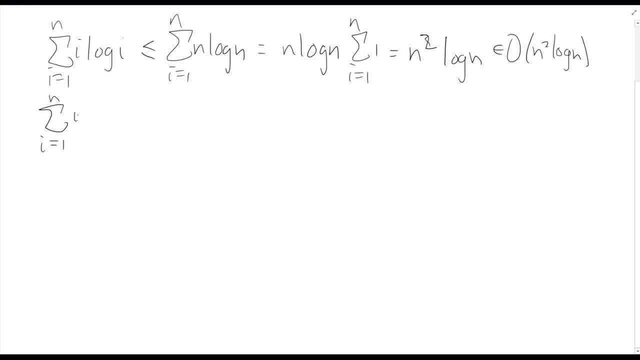 I don't like writing so much, And maybe you don't like writing so much either, And maybe you want to have a means of saving yourself a little writing. Now, one thing I don't want to write a lot because I know it's shown up in all our examples. 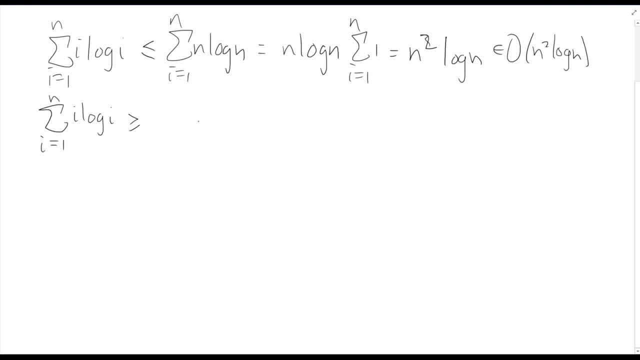 so far this floor of n over 2 plus 1, 4 of n over 2 plus 1.. I feel like I've written it a lot already. I'm going to have to write it some more And it's going to show up. 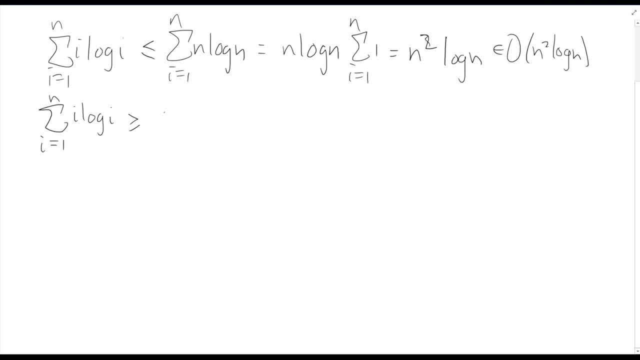 It's going to show up here in this i and in this i. I don't really want that. So, instead of using the floor of n over 2 plus 1, I'm going to use a technique we're always able to use. 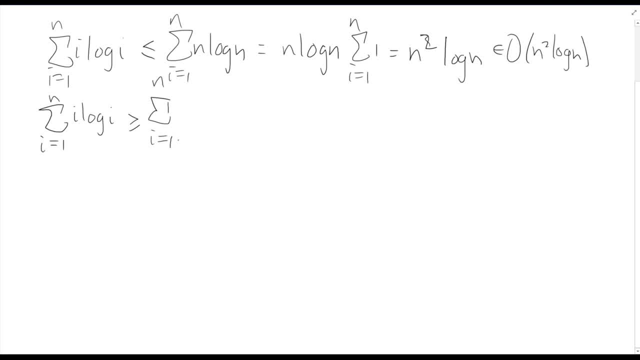 Oops, I put a 1 here, But this is fine, because what I really want is a k here. I want the value that I'm starting off at at k. Now, what is k? Well, maybe I'll put over on the side here. 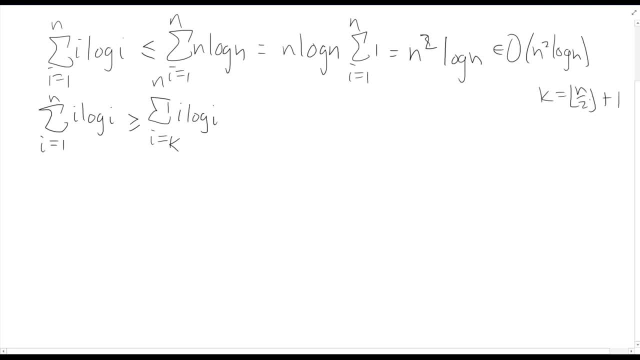 k is the floor of n over 2.. Plus 1.. Okay, Now I don't need to write it over and, over and over again. Let's continue with our approximation. then We've split the sum where I haven't really said, but it's at k. 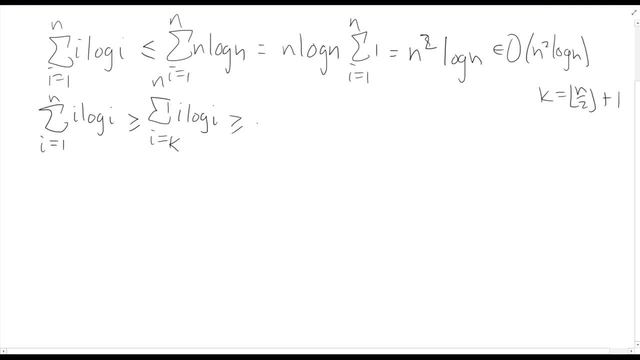 Over here I said what k was. So the next step: I'm going to swap out for k. All right, So now we have k log k instead of i log i Again. we can continue now with maybe a little bit of algebra. 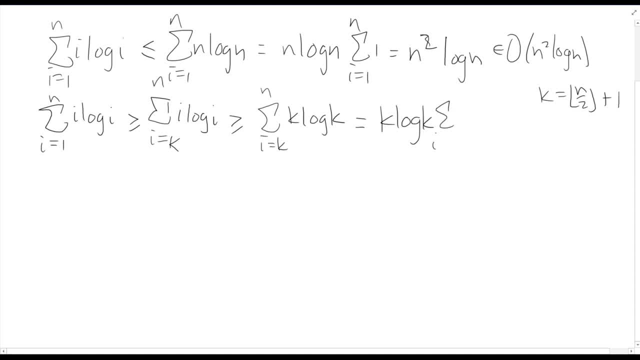 k log k. i equals k. So that's the sum. i equals k to n 1.. All right, Now what this sum is equal to. let's- yeah, let's take it one step further. We're going to get k log k times now. we need to be careful here. 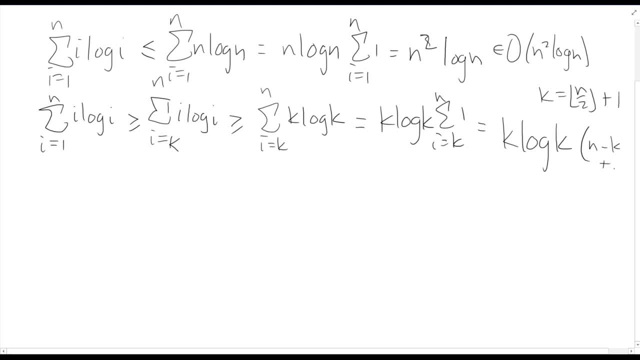 This one's going to be n minus k plus 1.. Okay, n minus k plus 1.. Remember, upper bound minus lower bound Plus 1 more. All right, Now we probably need to write all the nastiness back in there. 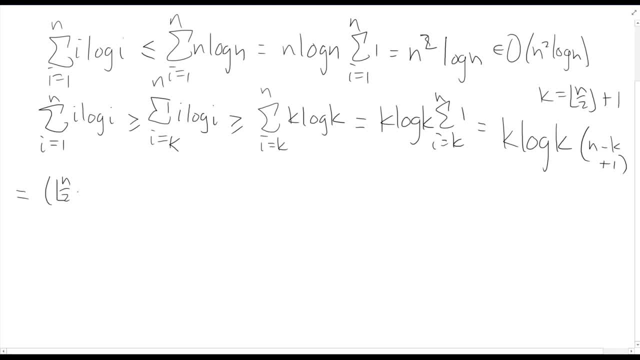 So let's go ahead and do 4 of n over 2 plus 1.. That was the first term out front. That's my first k. Okay, Now log. oh okay, 4 of n over 2 plus 1 here as well. 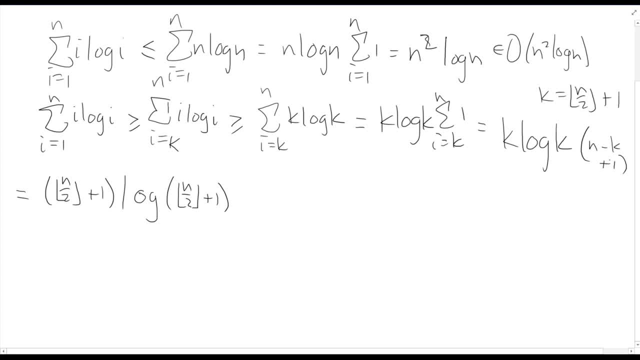 Okay, And then this next term. Well, this one I'm going to maybe cheat a little bit. I know I've got my floor of n over 2 plus 1 here. That's going in for my k. Well, then, the minus 1 that comes. 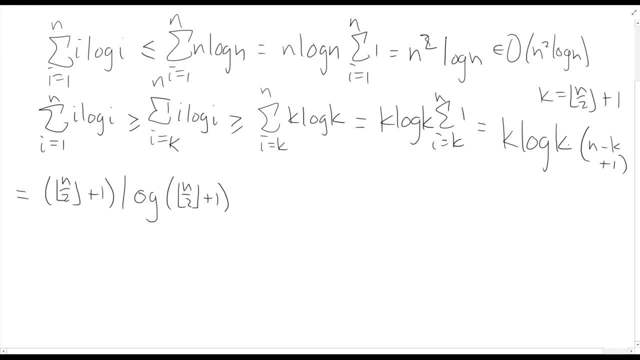 out of that cancels with my plus. I've got n minus the floor again. Oh well, that's that sum. we've already seen a few times, So again, if we've already seen it, we maybe know that that's the ceiling of n over 2.. 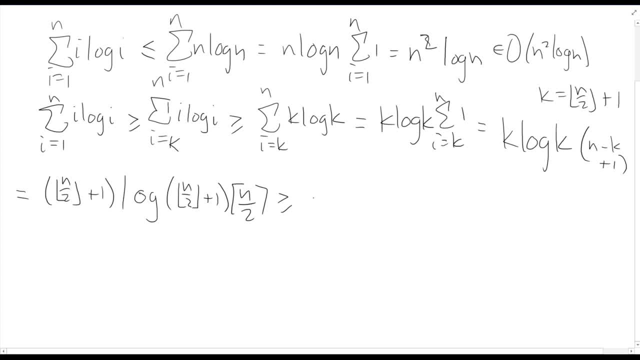 We still need to get rid of those floors and ceilings, And let's remind ourselves again that the ceiling we can overproximate away by just n over 2 itself. Next up, we have this one, this floor of n over 2 plus 1..